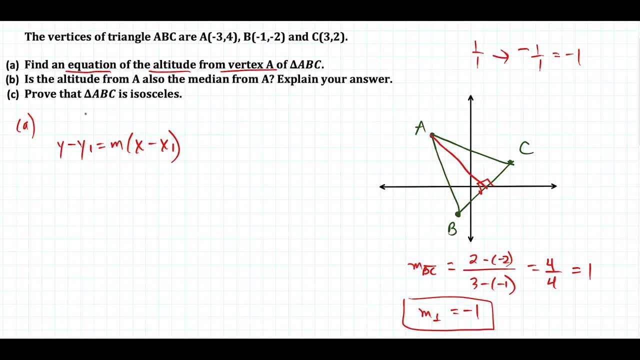 equals m times x minus x one, And we have the slope that we're going to use. we're using the slope negative one, And the point that we're going to use is negative three, four, because, remember, altitude is coming from vertex A. So A is definitely a point on our line that we need. 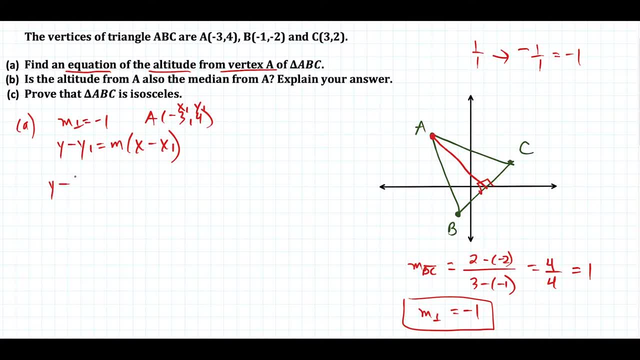 to write the equation of: So now we have y minus y one is equal to four equals, the slope is negative one. And then we have x minus negative three. But if I do minus negative three, this is going to change to plus three, So we'll just write x plus three inside parentheses here. And then we have y. 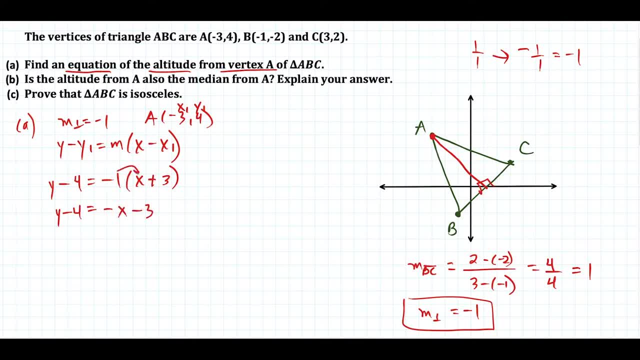 minus four equals negative x minus three. if we distribute this negative and then just add four to both sides And the equation of our altitude is going to be negative three, And then we have y minus x plus three, And then we have y plus negative x plus three, And then we have y minus x plus. 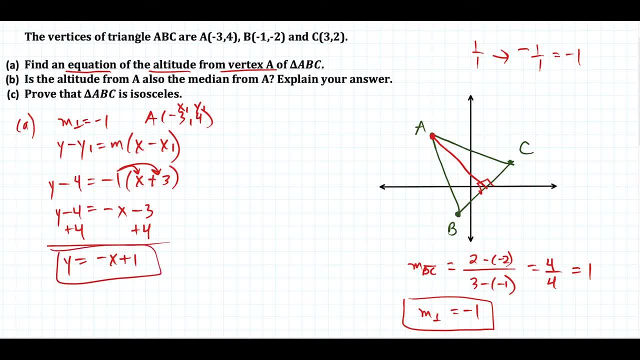 three, And then we have y minus x plus three, And then we have y minus x plus three, And then we have negative x plus one. So this answer is part A. For part B, what we want to do is we want to. 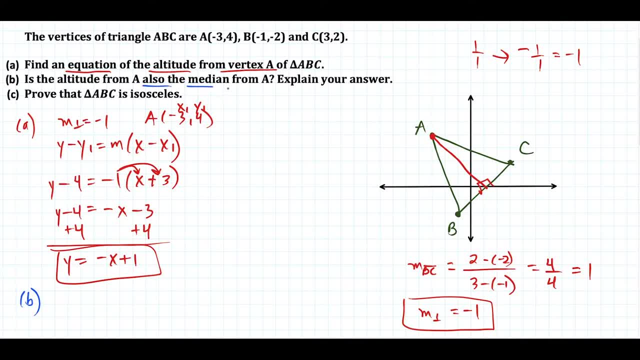 answer. the question is the altitude from A, also the median from point A. Well, just know, the median of a line segment, or, I'm sorry, the median of a triangle, is a line segment that goes from one vertex to the midpoint of the opposite side. So the question we really need to answer in B is: 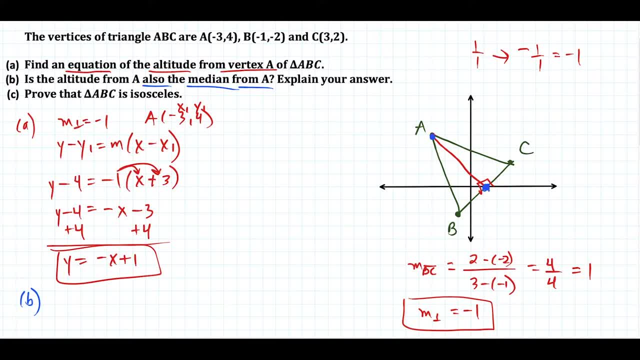 the midpoint of side BC is that point on the line y equals negative x plus one. So the first thing we'll do is find the midpoint of BC. And to find the midpoint what we do is we add the x coordinates together. we have negative one plus. 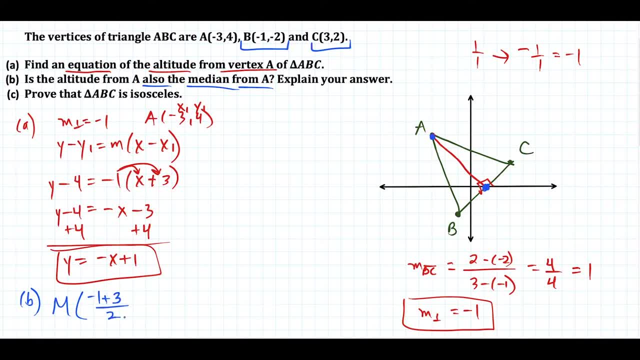 three make that a little neater. So we have negative one plus three, we're dividing by two, And then the y coordinate would be the sum of the y values: negative two plus two, dividing that by two. And when we simplify this we have four divided by. I'm sorry. 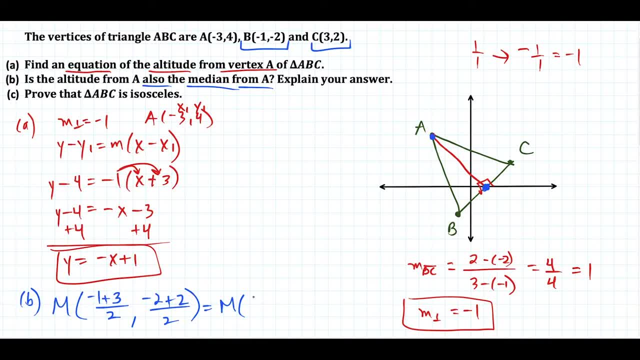 we have two divided by two- I almost forgot how to add- we have two divided by two is one and we have zero divided by two is zero. So the midpoint is one zero which is supported by the graph. But remember, formulas are way more reliable than graphs. 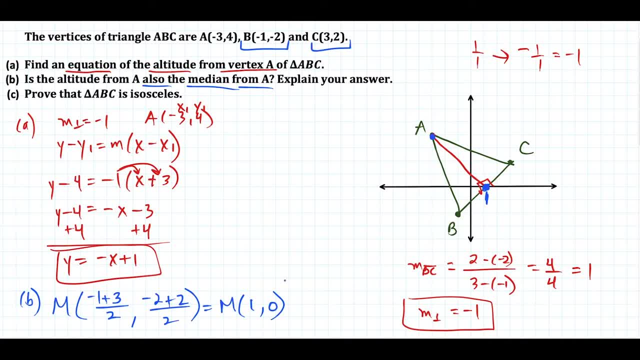 the graph is just there to kind of help us with the concept. So here's our midpoint. And remember, the question we have to answer here to establish that the median is also an altitude, is we have to answer: if one zero is a point on the line y equals negative x plus one. So to verify that, 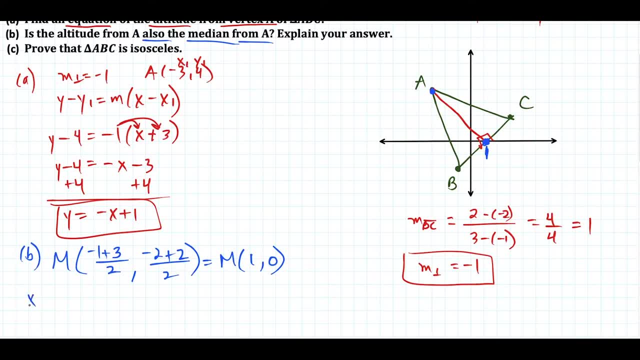 all we're going to do is just substitute. we have the midpoint has an x coordinate of one and a y coordinate of zero, And if we substitute that, if we substitute this into the equation of our altitude, we have zero equals and then we have negative one plus one. 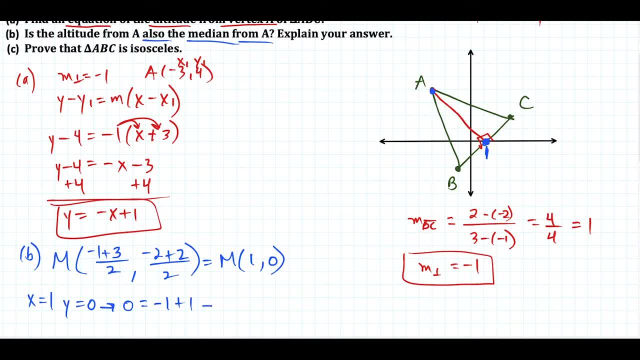 we're just replacing y with zero and x with one, And this gives us the equation zero equals zero, which is true it checks out. So now we can write a concluding sentence. we could say that the altitude is also a median, because the midpoint of side BC is on the line. y equals negative, x plus one. 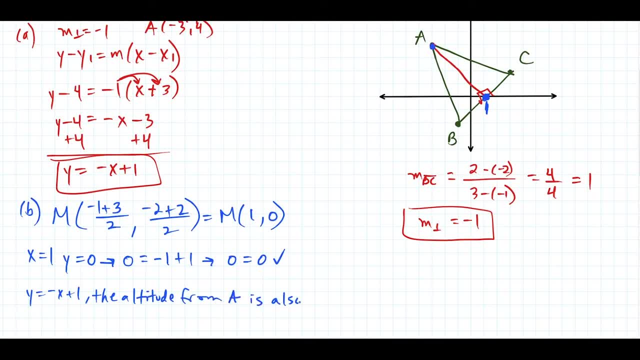 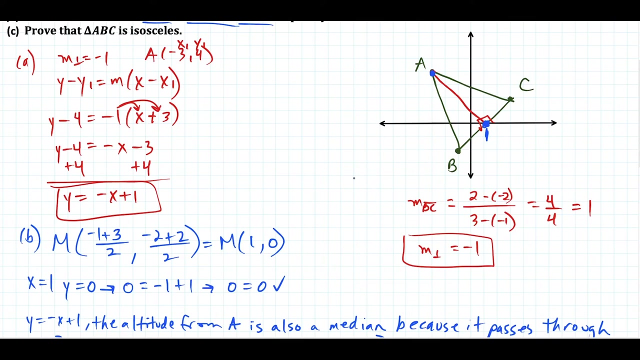 Okay, so this sentence here establishes that our line y equals negative. x plus one is an altitude and a median. So now the last thing that we have to answer here is: we have to prove that this triangle ABC is isosceles. But now we did the bulk of the work. 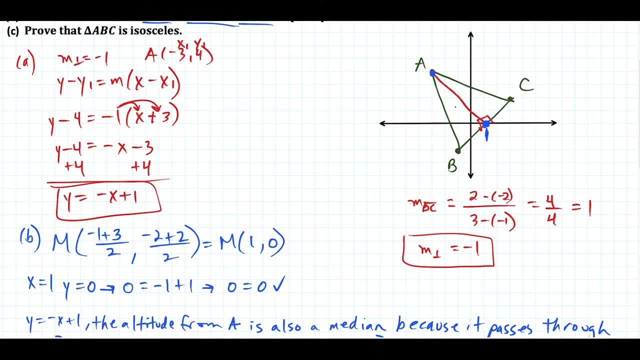 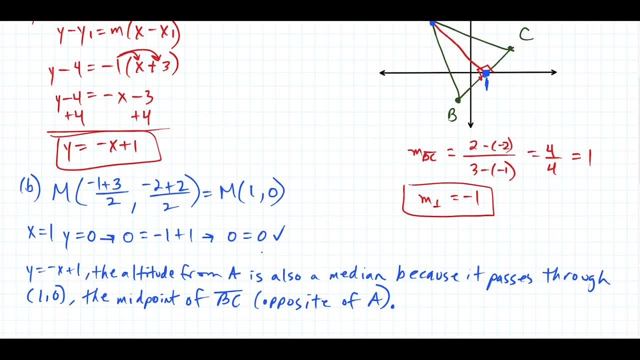 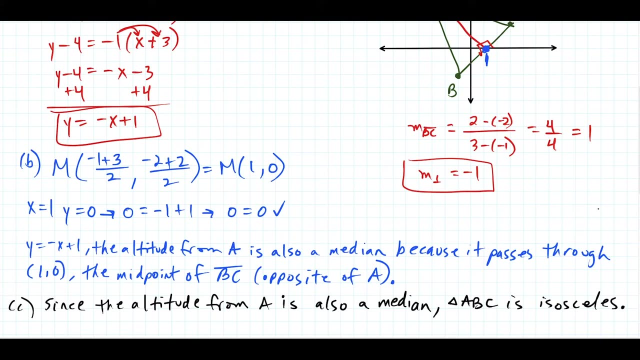 there's a very helpful theorem that says that if the altitude of a triangle is also a median, then the triangle involved is isosceles. So we could just write our concluding sentence Now. if this theorem was not known to you, there is also another way we could answer this, So we'll just look at an alternate. 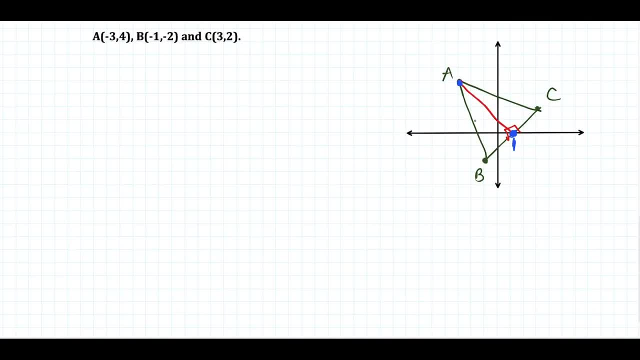 way of answering Part C. So what we could do is, if we look at the picture, we notice that AB and AC are the two sides that are equal in length. So another way of establishing that this triangle is isosceles is we could find the length of both sides and 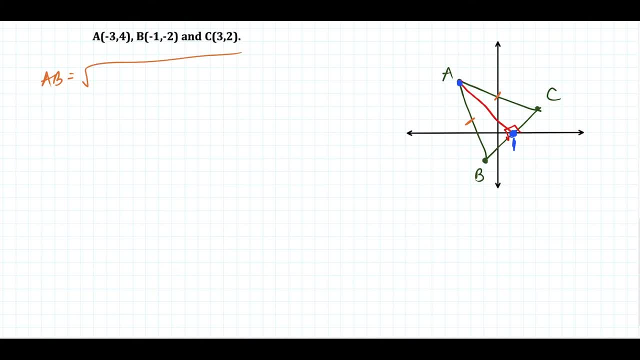 show that the lengths are the same. So if we use the distance formula here, we want to find the length of segment AB. we're doing the difference of the x coordinates. So we have negative three minus negative one, in parentheses, squared plus and then we have the difference of their y.